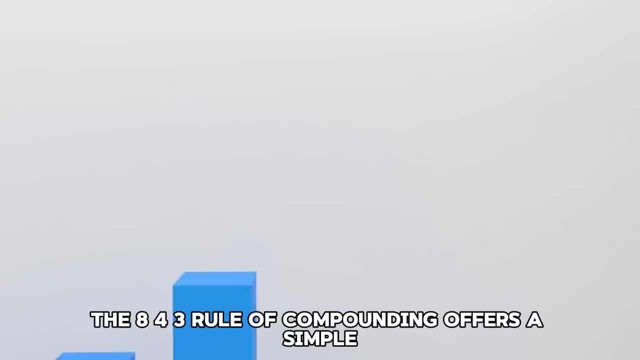 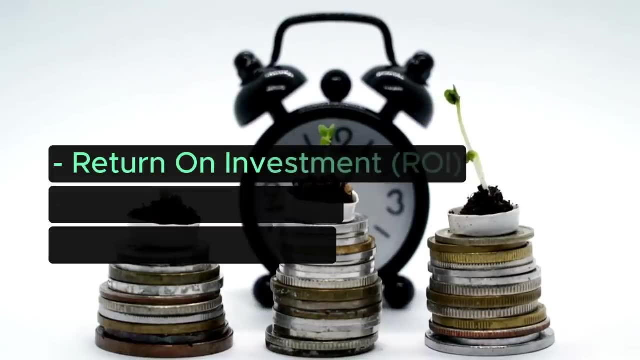 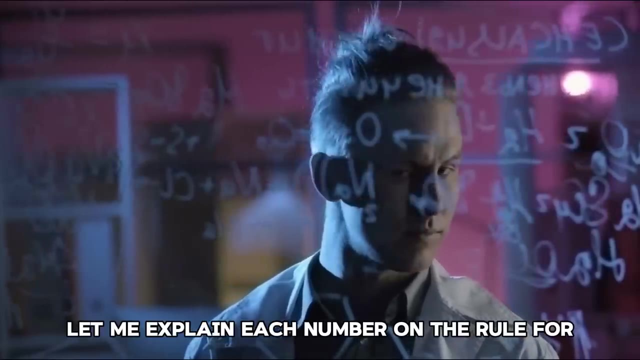 The 8-4-3 rule of compounding offers a simple yet powerful framework for wealth building. It involves three key elements: return on investment, investing duration and the number of assets to invest in. Let me explain each number on the rule for easier understanding. 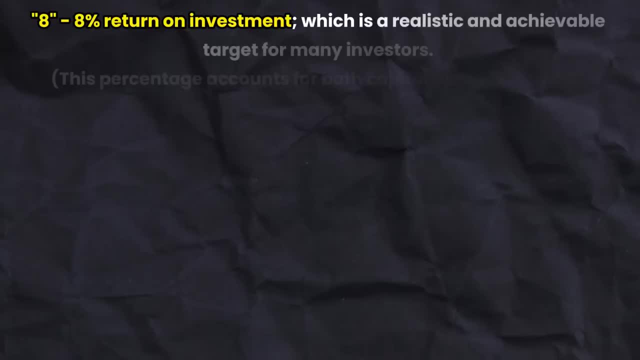 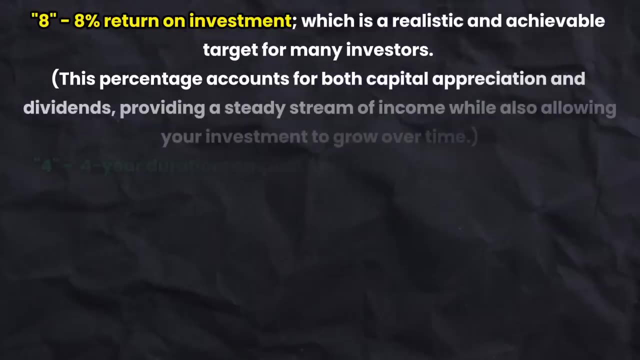 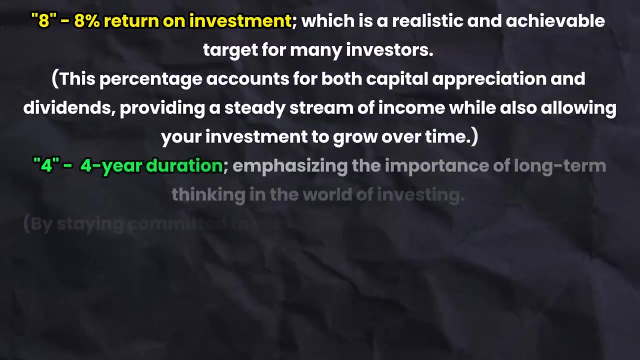 The 8 represents an 8% return on investment, which is a realistic and achievable target for many investors. This percentage accounts for both capital appreciation and dividends, providing a steady stream of income while also allowing your investment to grow over time. The 4 signifies a 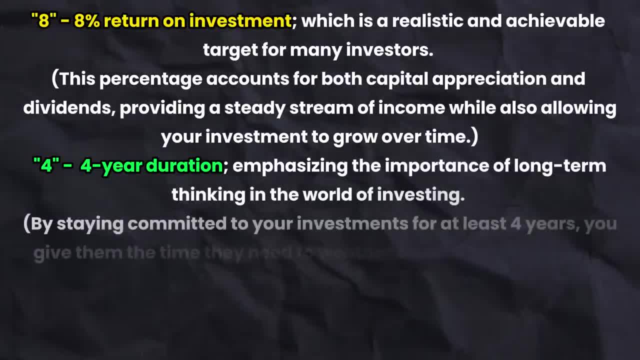 four-year duration emphasizing the value of your investment over time. The 4 signifies a four-year duration emphasizing the importance of long-term thinking in the world of investing. The 4 signifies a four-year duration emphasizing the importance of long-term thinking in the world of investing By staying committed to your 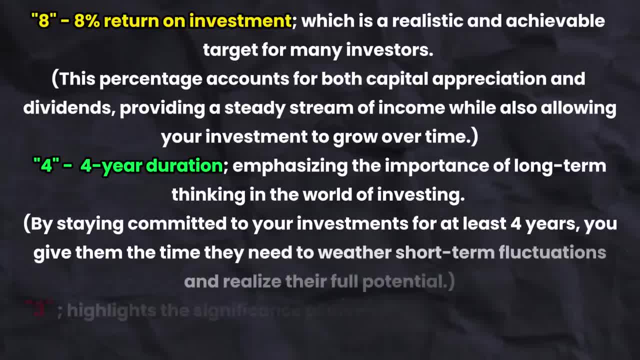 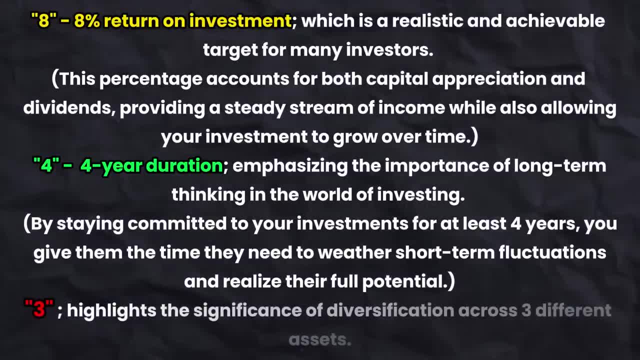 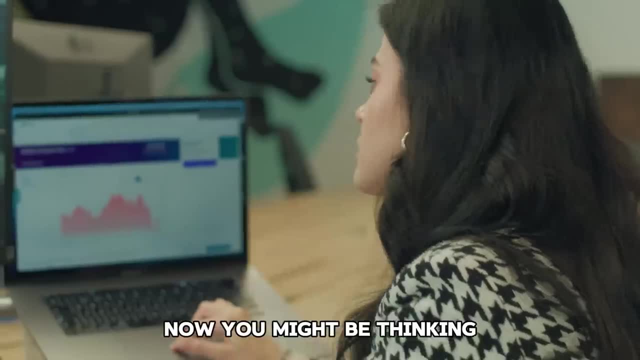 investments for at least four years. you give them the time they need to weather short-term fluctuations and realize their full potential. Finally, the 3 highlights the significance of diversification across three different assets. Now you might be thinking: why invest in three? 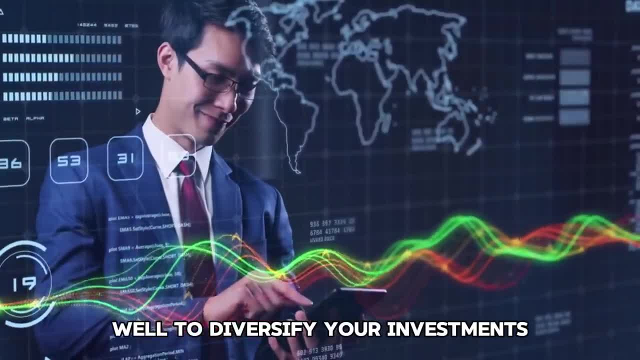 assets Well to diversify your investments by spreading the wisdom and gifts of the Financier. I had an opportunity to share a few tips on what are the best ways to invest. You may have issues in news spreading them across different assets to reduce your risk and increase your chances of long-term. 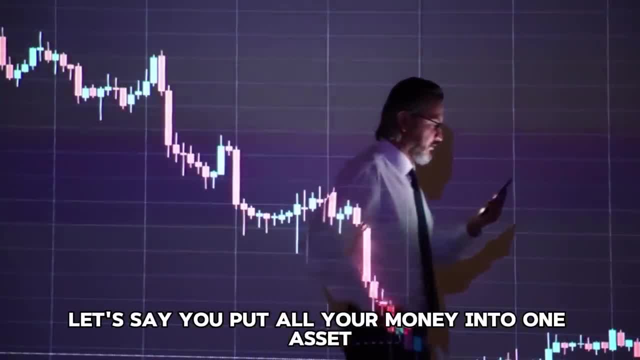 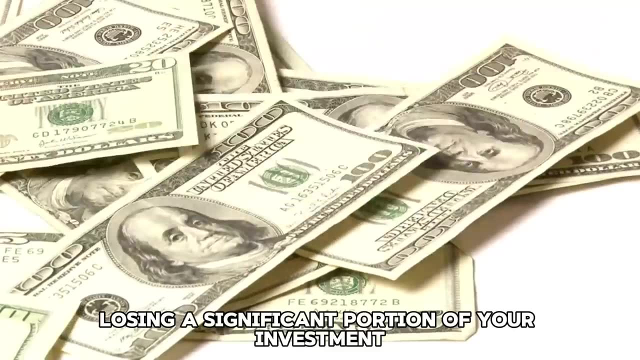 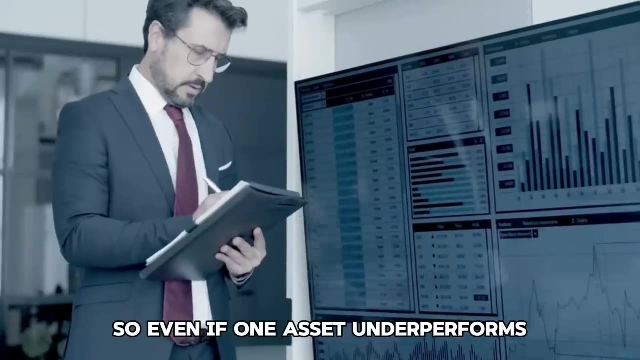 success. Let's say you put all your money into one asset like the stock market, and it doesn't perform as expected. You could end up losing a significant portion of your investment. But by diversifying you're not putting all your money in one investment. So even if one asset 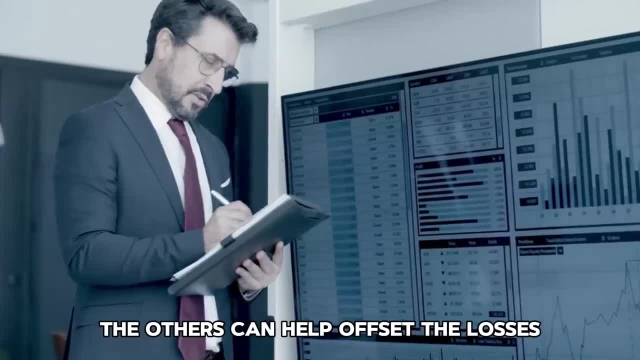 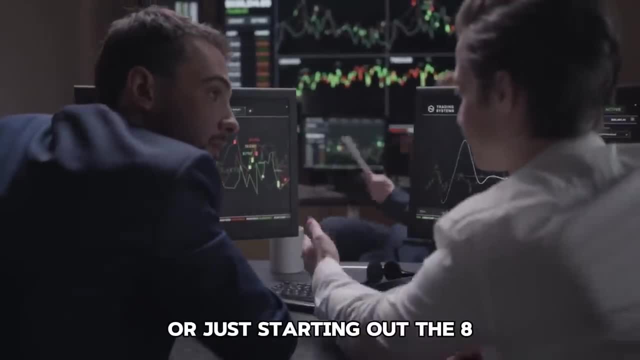 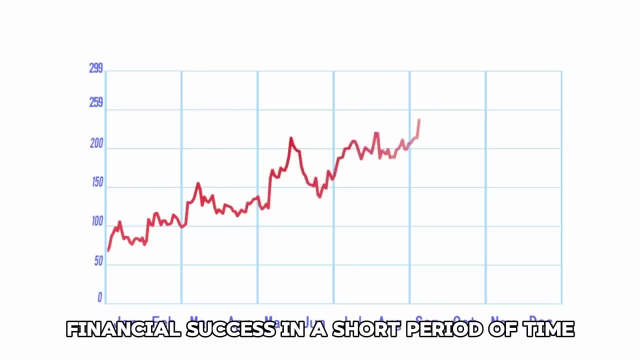 underperforms, the others can help offset the losses, keeping your overall portfolio more stable. So, whether you're a seasoned investor or just starting out, the 8-4-3 rule provides a clear roadmap for achieving financial success in a short period of time. To understand how this works, 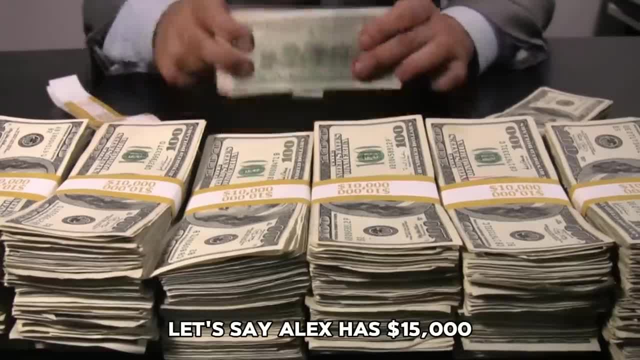 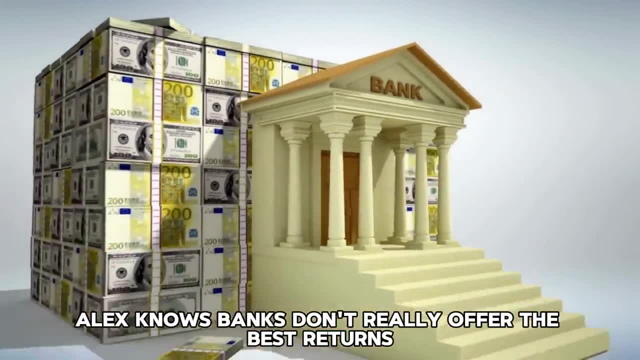 let's look at an example. Let's say Alex has $15,000 now lying in his bank account. Alex knows banks don't really offer him any money, So he's going to put all his money in one asset to offer the best returns. So he decides to divide the money equally and invest it in three. 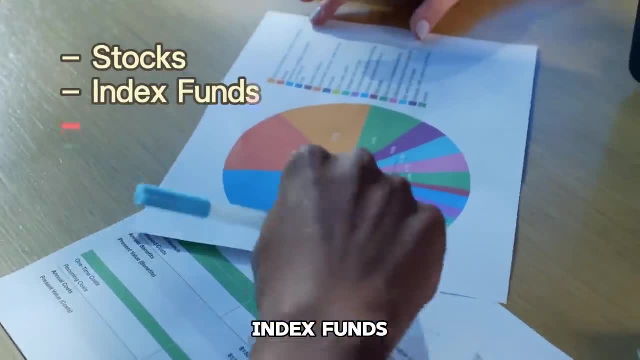 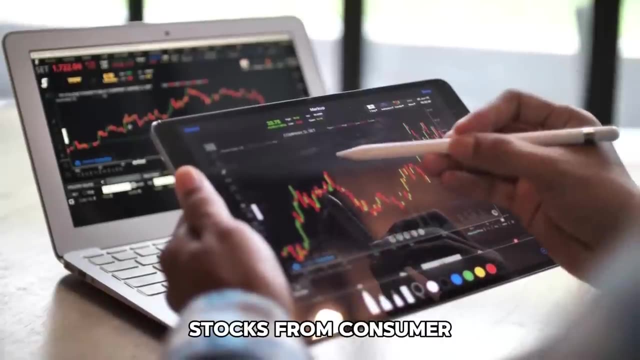 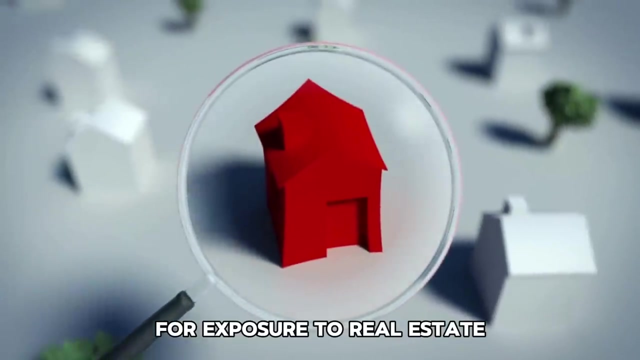 assets. These are stocks, index funds and real estate investment trusts. Index funds representing the broader market stocks from consumer-stable or tech companies, and real estate investment trusts for exposure to real estate Over the course of four years, assuming an average annual return of 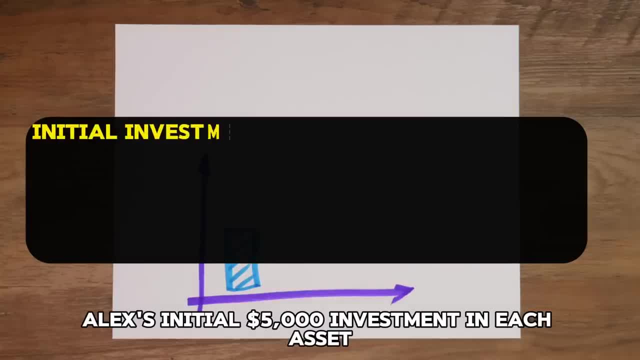 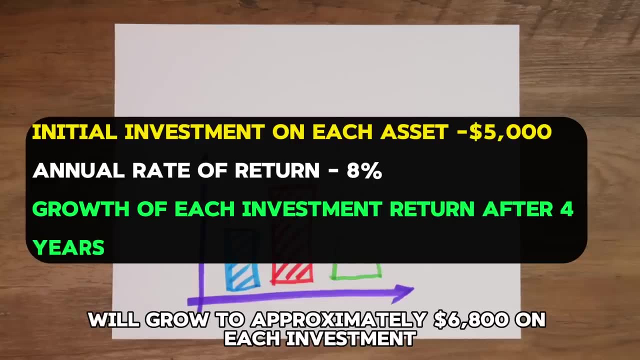 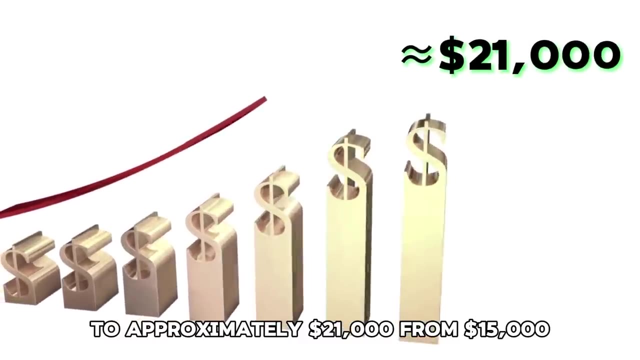 8% for each asset. he decides to divide the money equally and invest it in three assets. Alex's initial $5,000 investment in each asset will grow to approximately $6,800 on each investment, adding up his total final investment after four years to approximately $21,000 from. 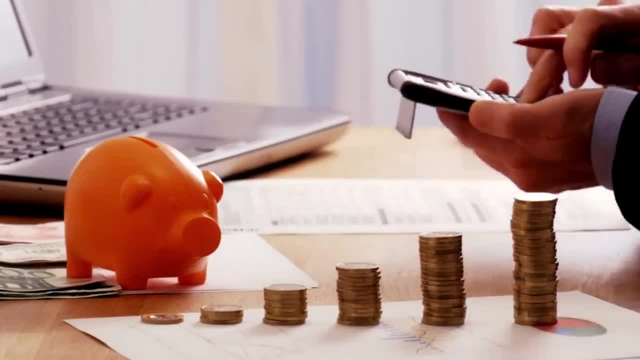 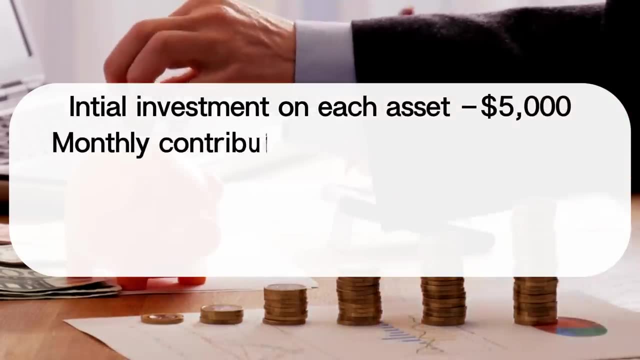 $15,000.. In another scenario, let's say Alex commits to a disciplined monthly contribution of $500 to each asset. After four years, Alex's initial $5,000 investment in each asset will grow to approximately $34,000.. Each of his assets will have grown by 8%, resulting in each of his 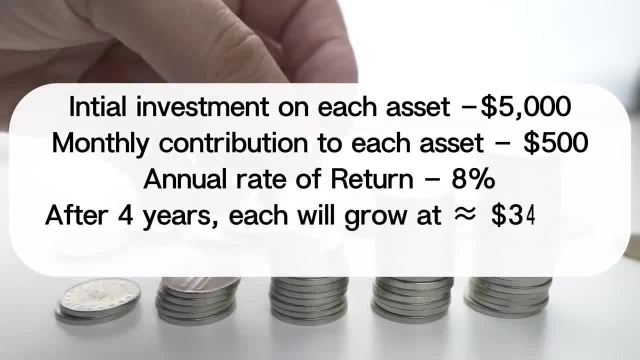 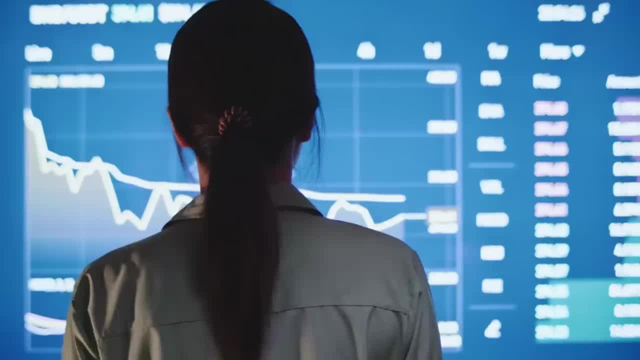 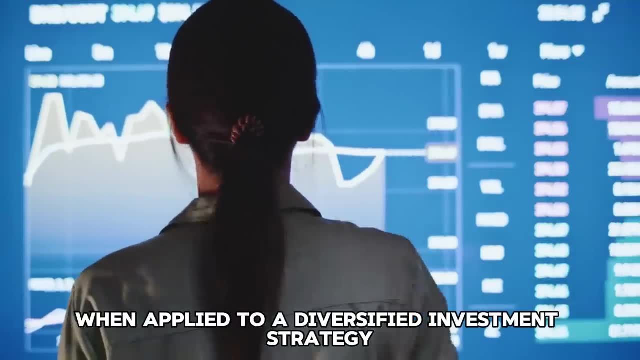 investments being valued approximately at $34,000, adding up the total value of the three investments to over $102,000,, showcasing the remarkable potential of the 8-4-3 rule when applied to a diversified investment strategy. Okay, so, now that we understand the 8-4-3 rule and the power, 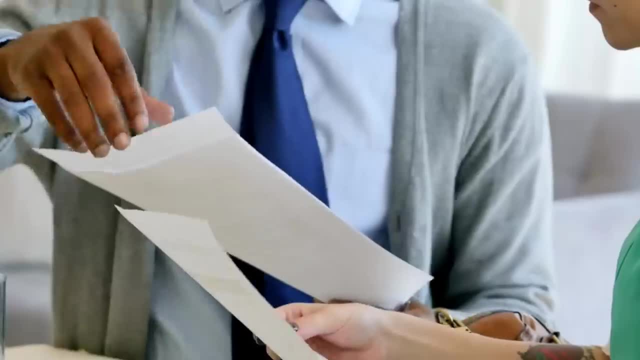 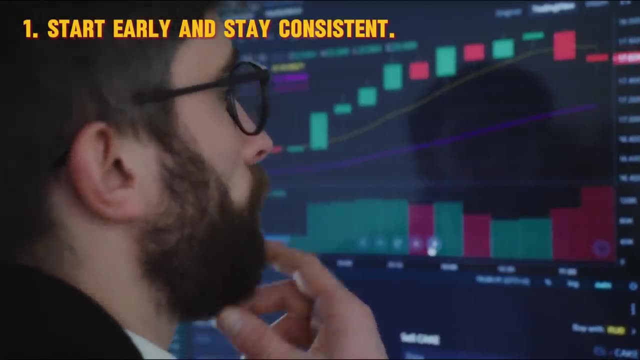 of compounding, how do we decide to divide the money equally and invest it in three assets? How do we put it into action? Well, by using the following simple principles of smart investing: 1. Start early and stay consistent. Starting early is crucial in the world of investing. 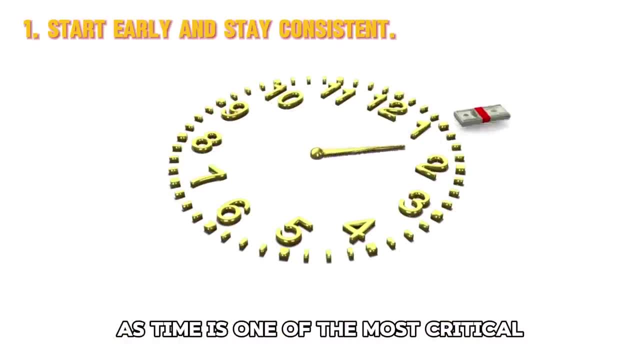 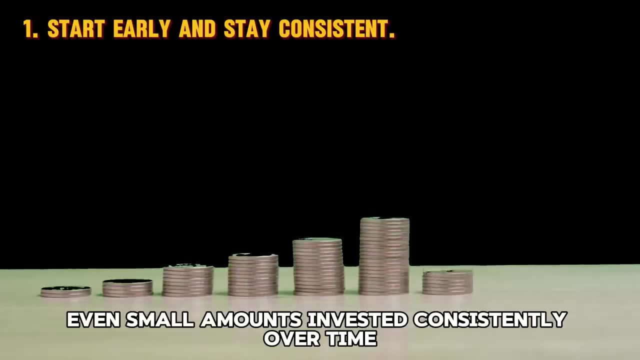 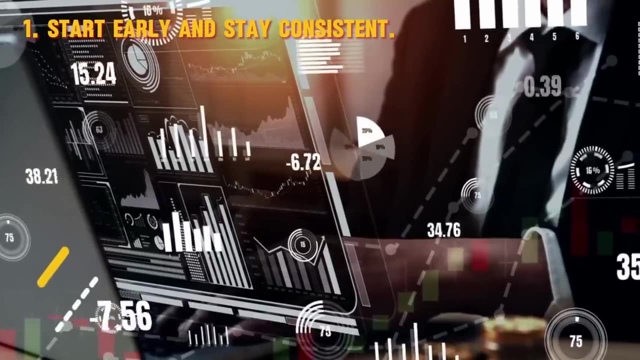 because of the power of compounding, as time is one of the most critical aspects of any investment strategy. Even small amounts invested consistently over time can grow into significant sums due to compounding effect. 2. By starting early, you give your investments more time to grow, which can ultimately lead to. 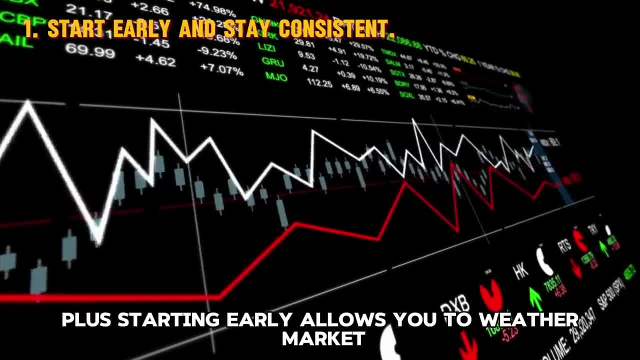 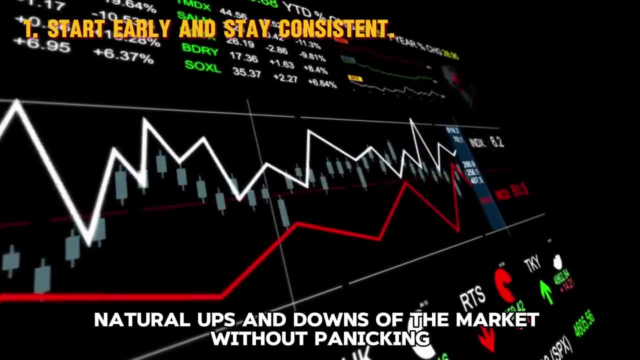 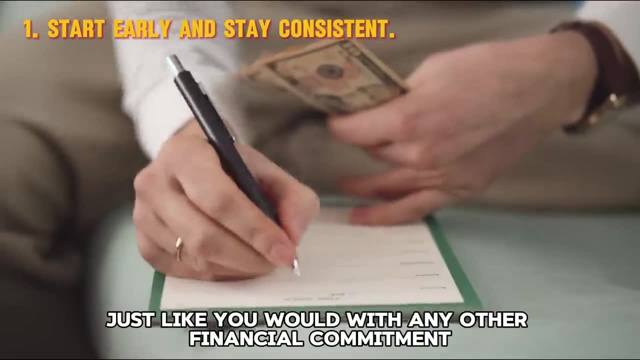 greater wealth accumulation in the long run. Plus, starting early allows you to weather market fluctuations and take advantage of the natural ups and downs of the market without panicking. Set a budget, stick to it and make investing a priority, just like you would with any other. 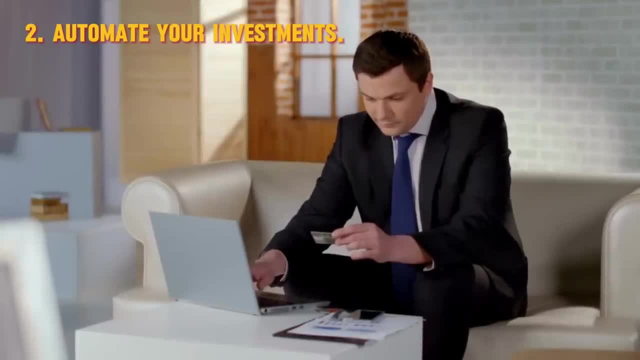 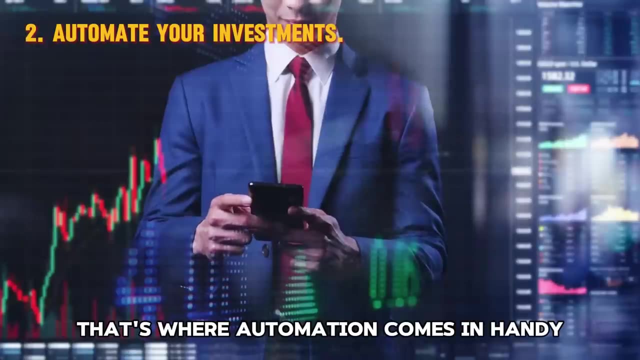 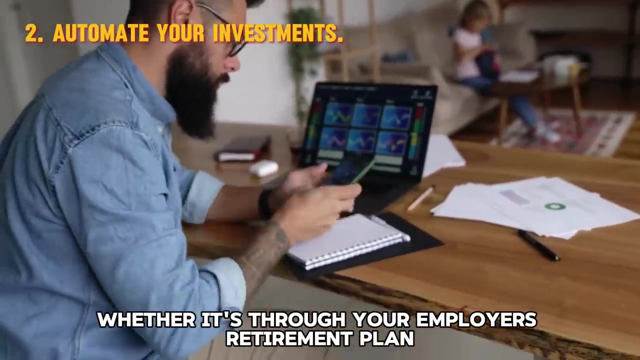 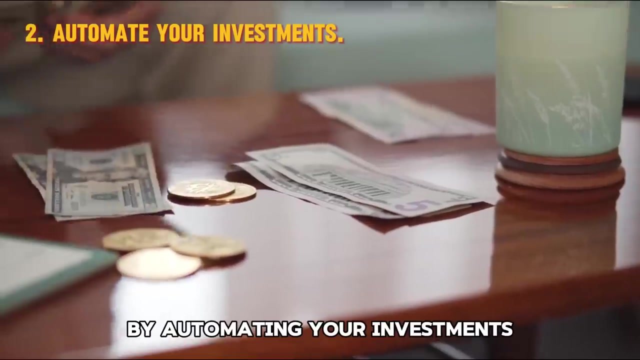 financial commitment. 2. Automate your investments. Life can get busy and it's easy to forget to invest regularly. That's where automation comes in handy. Set up automatic contributions to your investment accounts, whether it's through your employer's retirement plan, a brokerage account or a robo-advisor platform. By automating your 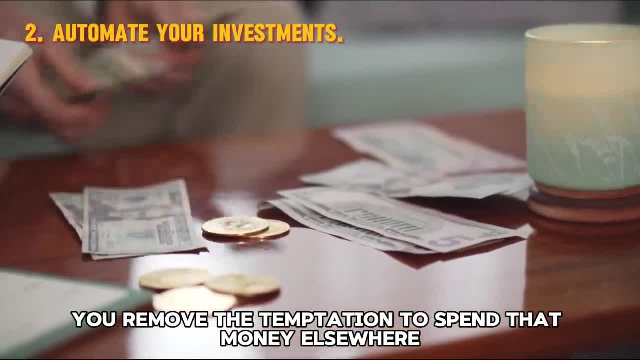 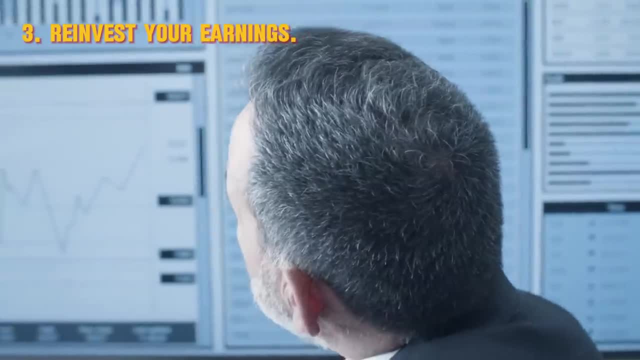 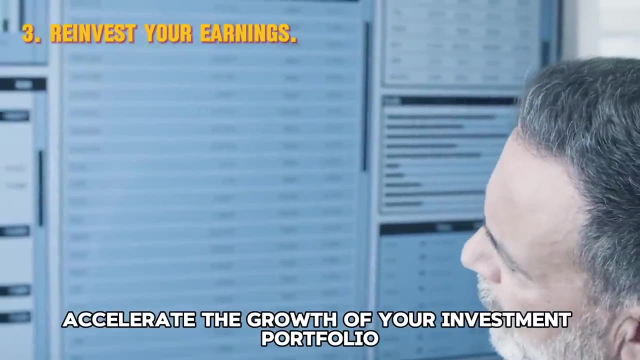 investments, you remove the temptation to spend that money elsewhere and ensure that you're consistently adding to your portfolio over time. 3. Reinvest your earnings. Reinvesting your returns is a powerful way to accelerate the growth of your investment portfolio. Instead of cashing out or pocketing your gains, reinvest them back into. 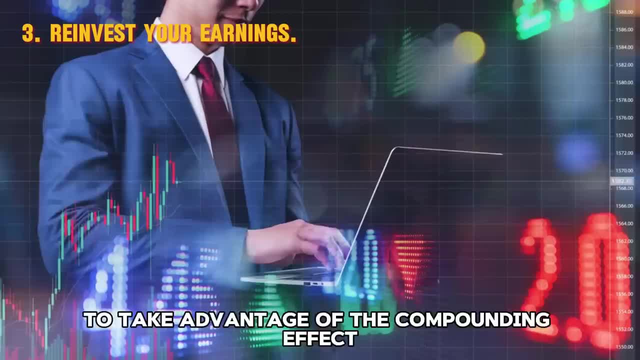 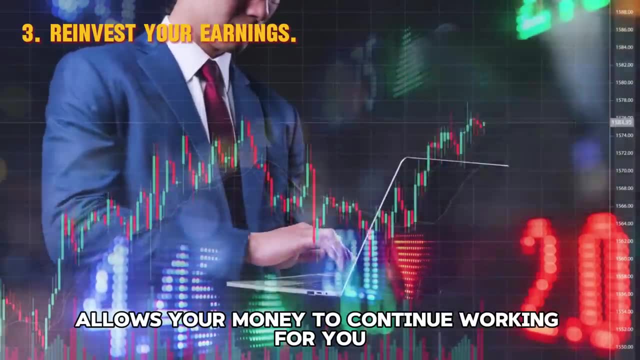 your portfolio to take advantage of the compounding effect. Reinvesting dividends, interest and capital gains allows your money to continue working for you, compounding over time and generating even greater returns. This simple yet effective way of investing can help you to. 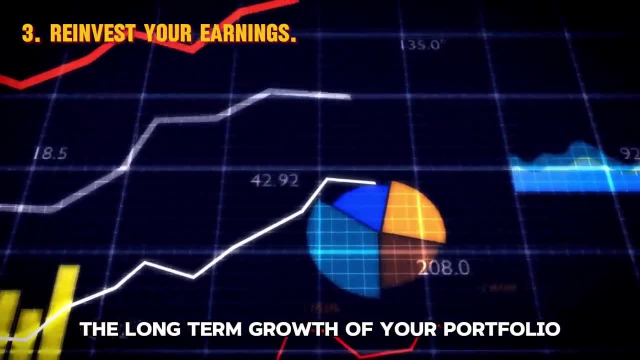 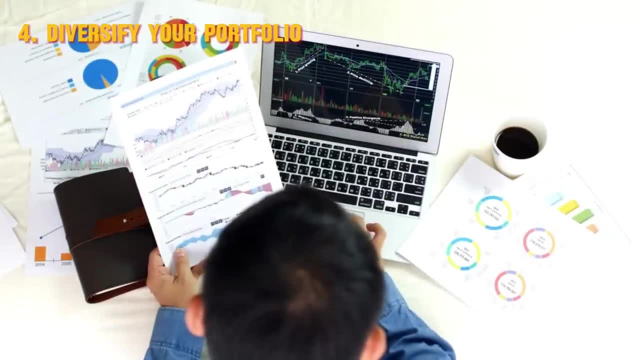 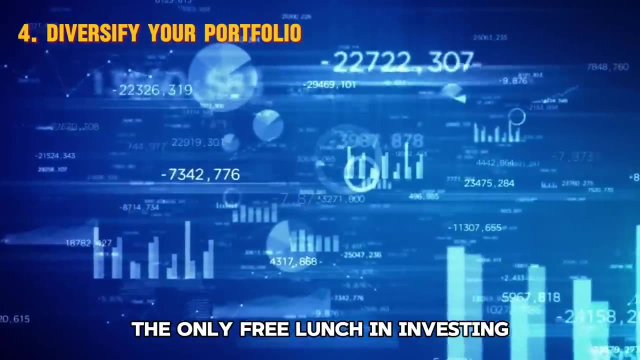 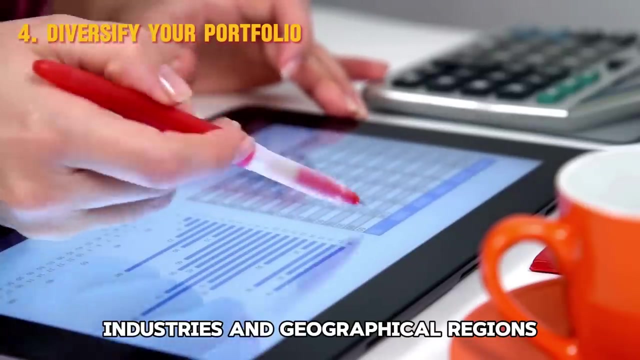 maximize your investment bonus and you become a value defender. 4. Diversify your portfolio. Diversification is often referred to as the only free lunch in investing. By spreading your investments across different asset classes, industries and geographical regions, you can reduce the overall risk in your portfolio. If one asset breaks down in a duty-based way, this means that PRACTICAL investing firms will return for profit. This is not something you can do immediately by making a profit. You have to start building your portfolio beforehand, and this is aesterisk to your growth. If you've done this, 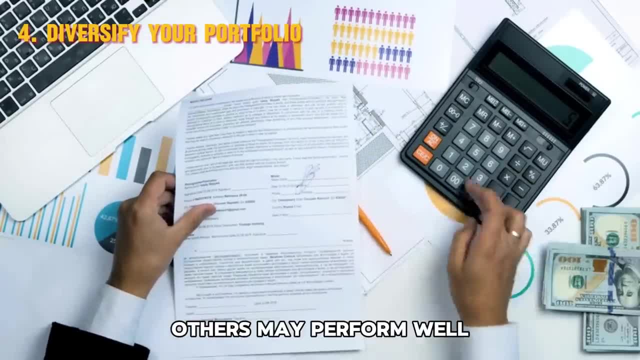 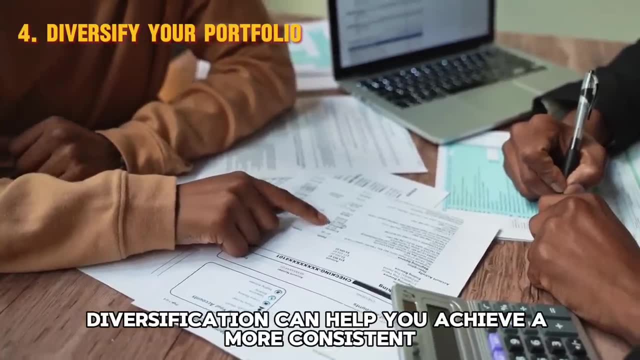 invest your savings. If you've invested in a long-term investment portfolio, increase your value by A to Z. One asset performs poorly, others may perform well, helping to offset losses and stabilize your overall returns. Diversification can help you achieve a more consistent and smoother investment journey, protecting your wealth over the long term. 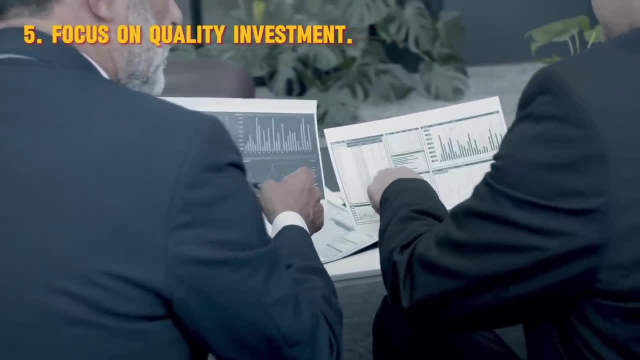 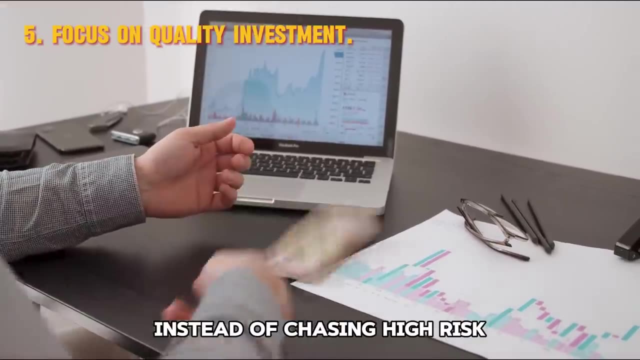 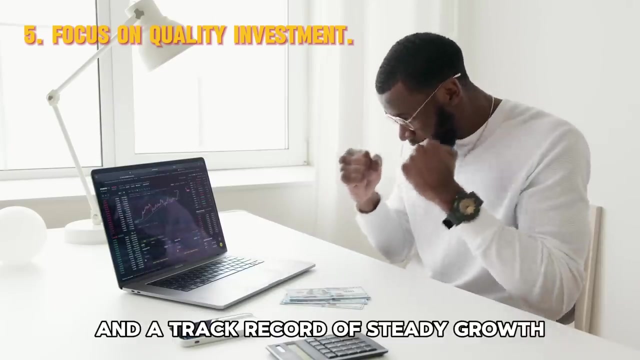 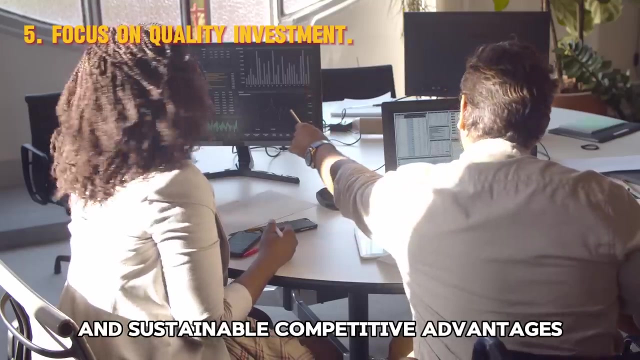 5. Focus on Quality Investment. Quality over quantity is a mantra that holds true in investing. Instead of chasing high-risk, high-reward opportunities, focus on quality investments with strong fundamentals and a track record of steady growth. Look for companies with solid financials, reliable cash flows and sustainable competitive advantages.